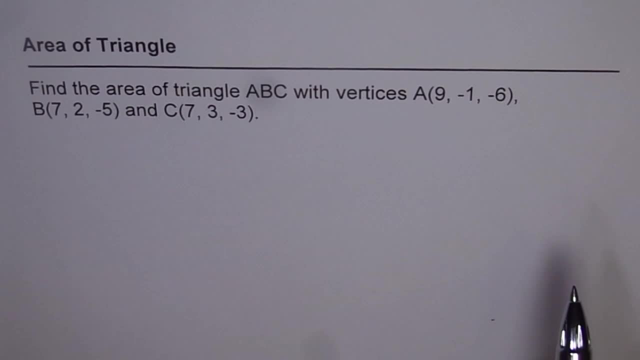 what are the vectors? A, B, B, C and C? A representing the three sides of the triangle, and then we can have cross product. The cross product will actually give us area of the parallelogram. that means two triangles. So to find area of triangle we should write: 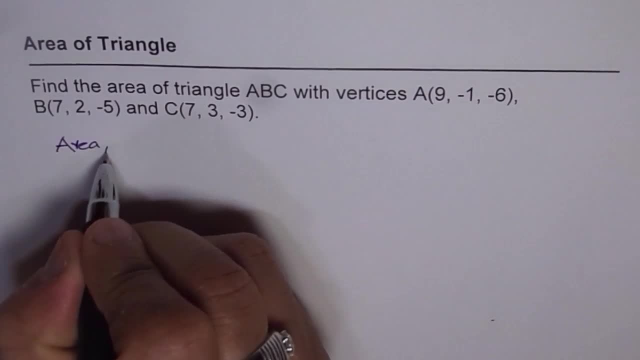 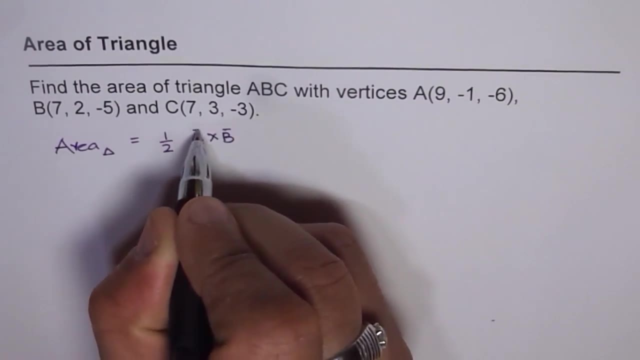 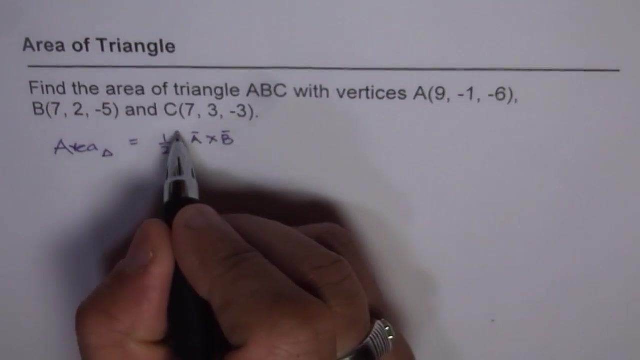 area of triangle is equal to half of A cross B. Now, remember we have to find the area of triangle. So to find the area of triangle, remember cross product is truly a vector. So we need to take just the magnitude of A. 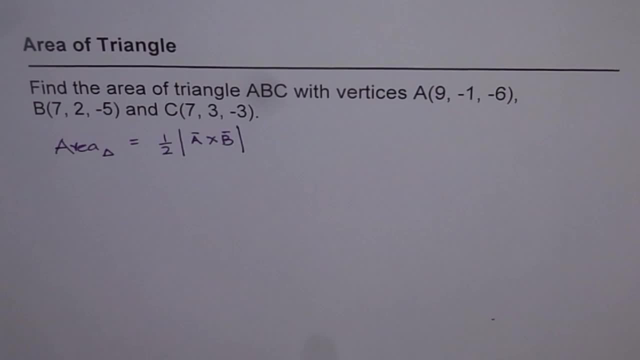 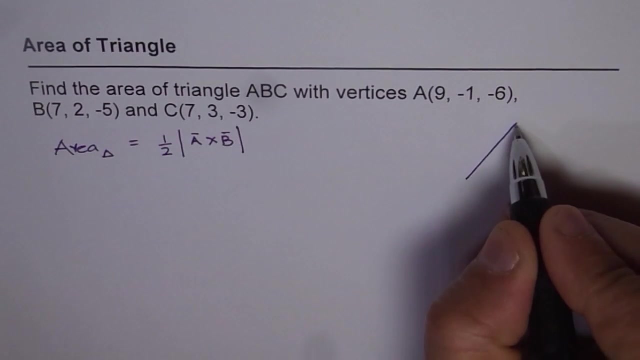 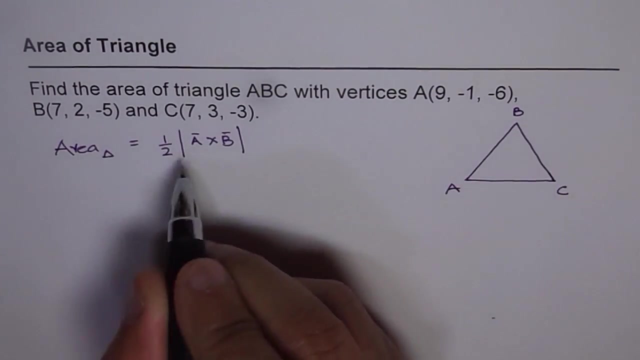 cross B. Now here, A is the side opposite to vertex A. that means I am saying side BC and B is the side opposite to vertex B. So let me just make this triangle once here and tell you what I am saying. Let's say this is A, B and C. Then when I say vector A, I am just saying referring to 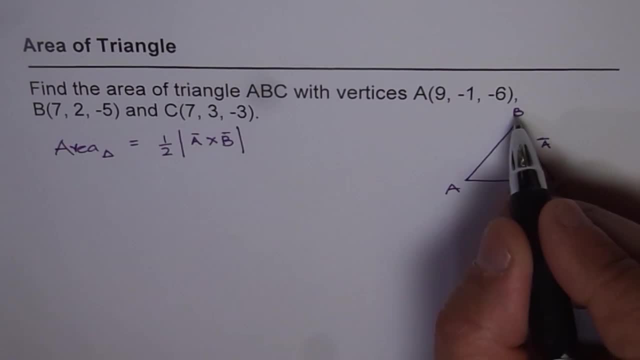 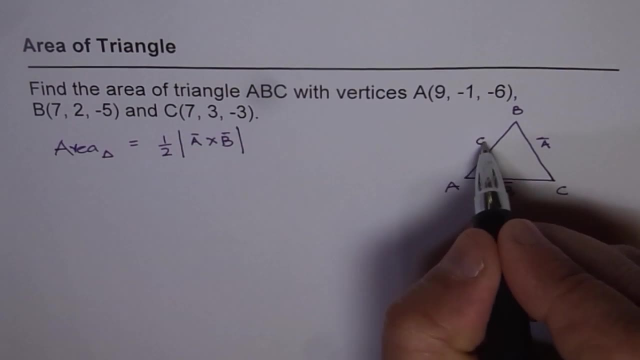 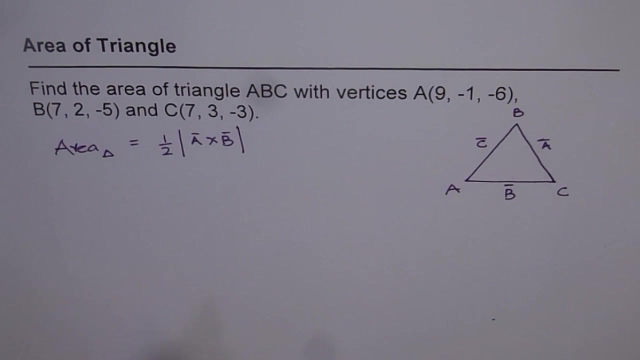 this side A, which is opposite to A, And when I am saying B, I am referring to the side opposite to B, and when I say C, it is referring to side opposite vertex C. So from this, have a look at this triangle. Anyway, you can find any two sides. So let's find side AC first. 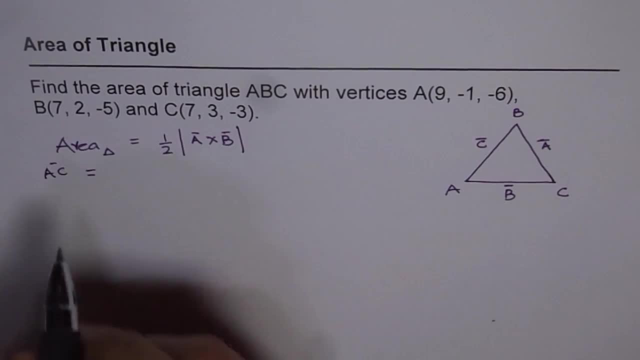 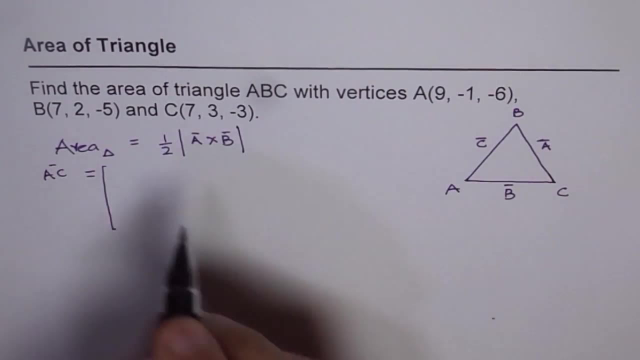 for example, AC is equal to A is here and C is there. So what we will do is I will use matrix here. So AC, C minus A. So write 7, 3, minus 3.. And A is 9 minus 1.. So we will take away those. 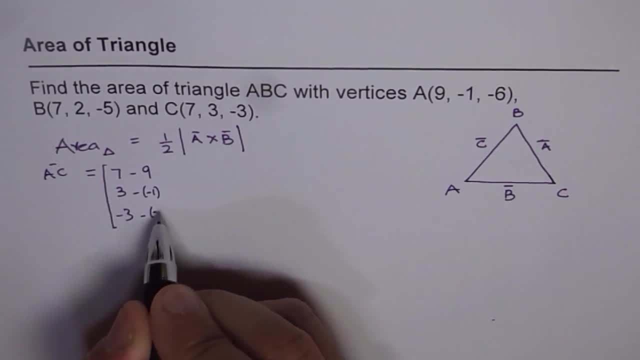 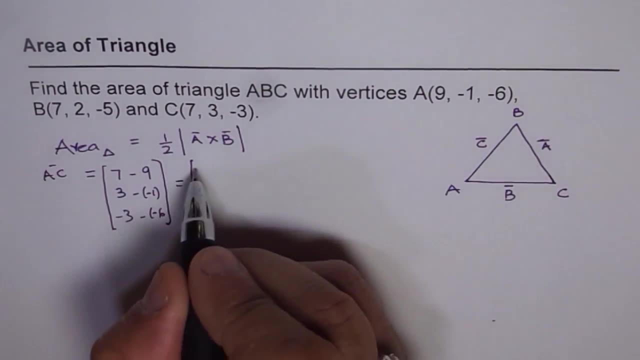 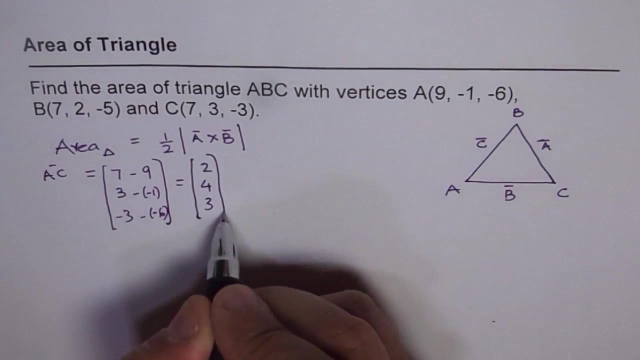 which is 9 minus 1 and minus 6, right, And that gives us AC, which is 7 minus 9,, 2, 3 plus 1, 4.. Minus 3 plus 6 gives us 3, right, So we get AC. Now. vector A is side BC for. 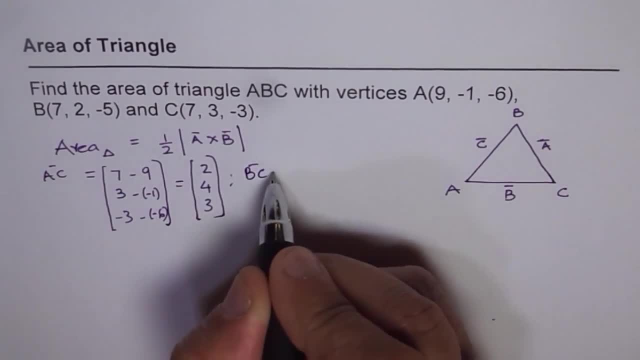 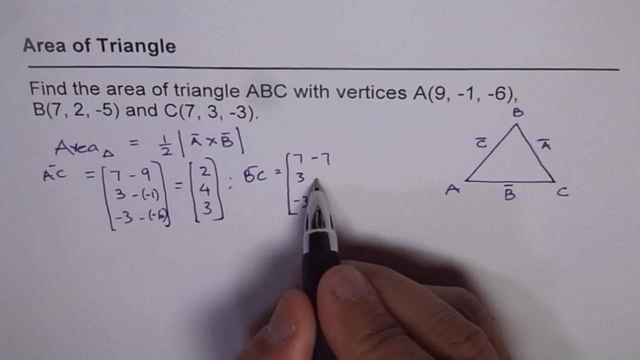 us. So we say: BC is equal to B to C. So we will say: 7, 3, minus 3.. 7, 3, minus 3. Minus of 7.. From here we will do: minus of 2.. And minus of minus 5 is plus 5.. So we will write. 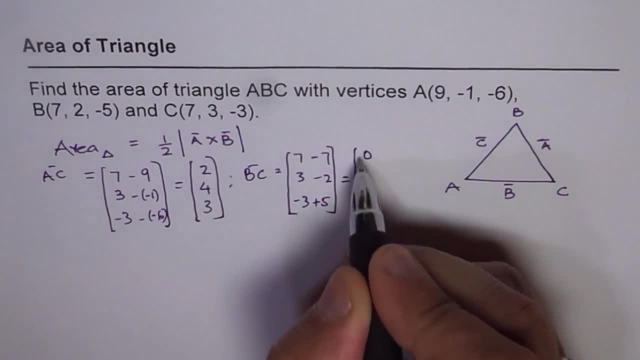 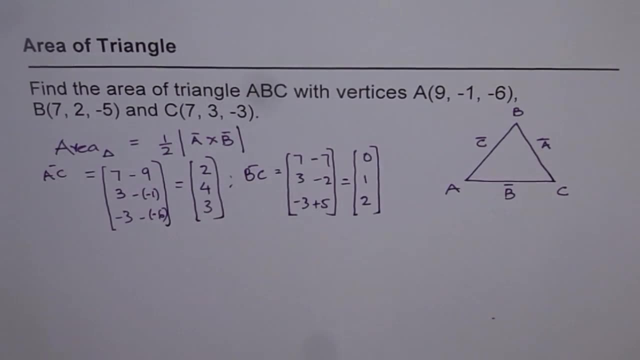 5. So BC is 0,, 1, and 2 for us. So you got AC and BC. Now area of the triangle is equal to half times cross product of. let me write now: AC cross, BC, right, And after doing the, 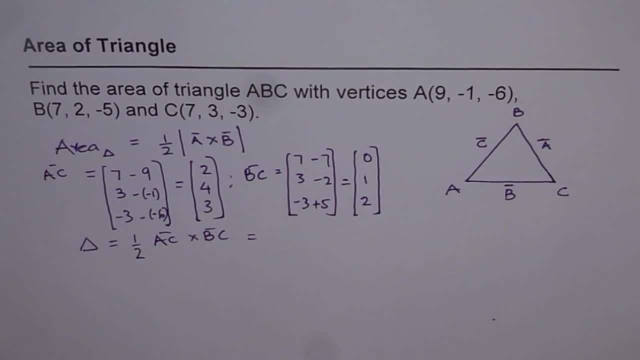 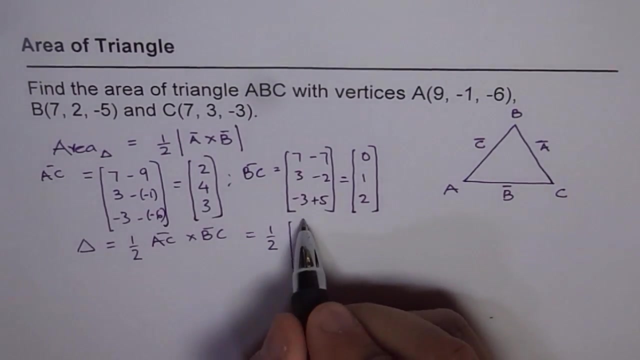 cross product. we will actually take the magnitude right. cost product is: half of AC is 243 and BC is 012.. So we can use the matrix method or we can use our rows method. Let's use matrix here, So we write the components: IJK, AC is. 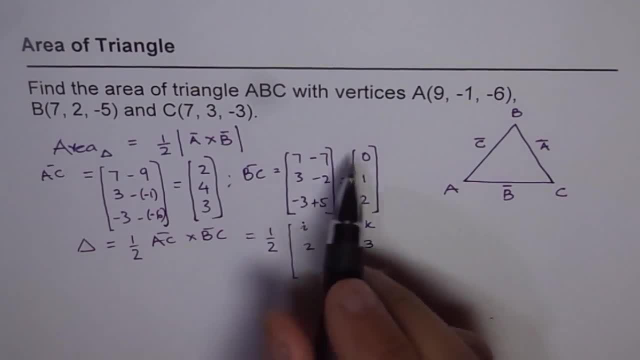 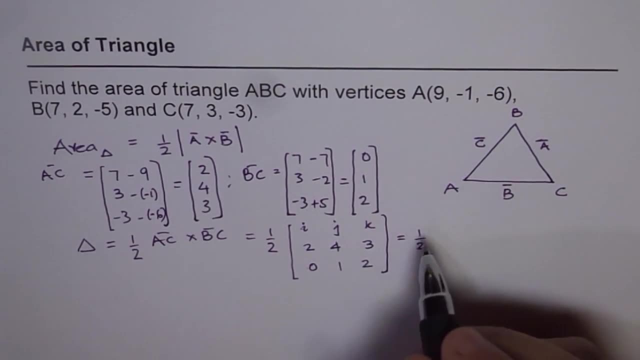 243 and BC is 012.. So it is equal to half of. let me put the brackets here Now. I component is 4 times 2, 8 minus 3 minus J. OHK is 243.. OHK is 243. 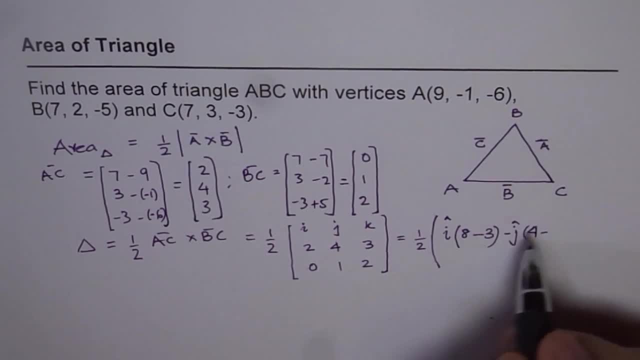 Which is 2 times 2, 4 minus 0, plus K, which is 2 minus 0. So just 2.. That's what it is. So we get our cross product as equals to. let me write it here now: half of 5I minus 4J. 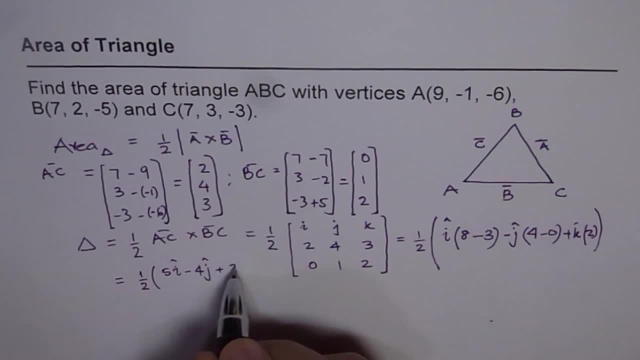 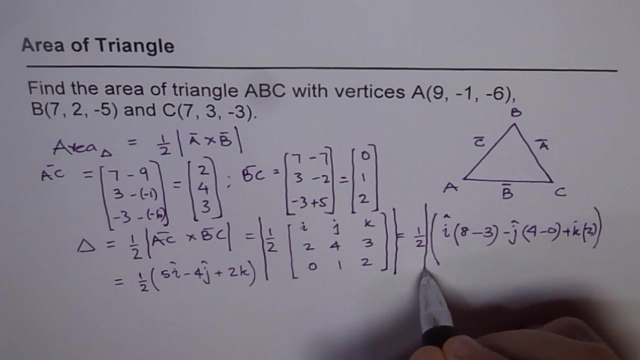 plus 2K. Now, area is the magnitude of this right. So we need to find area as magnitude of this vector. So what I will do is I'll write magnitude here. Okay, So that makes it complicated, but I hope you understand what I'm trying to say, And that is this. 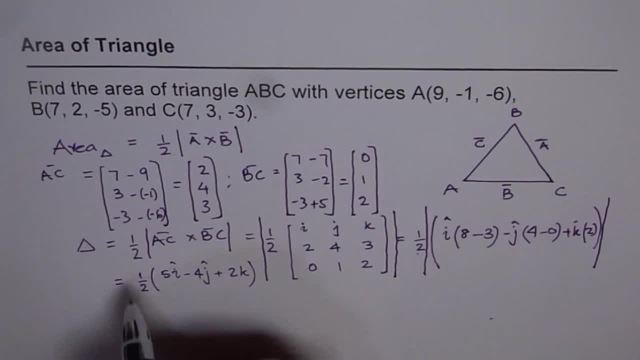